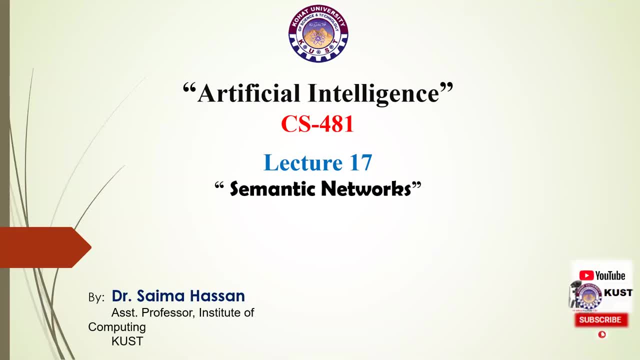 In order to solve various problems and to draw some conclusions. we often have information already stored in our brain that we can utilize. But how is that information stored in our brain? There are a lot of possibilities. Today, we are focusing one of them, which. 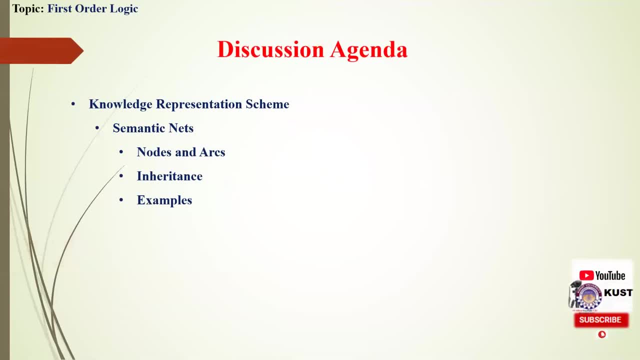 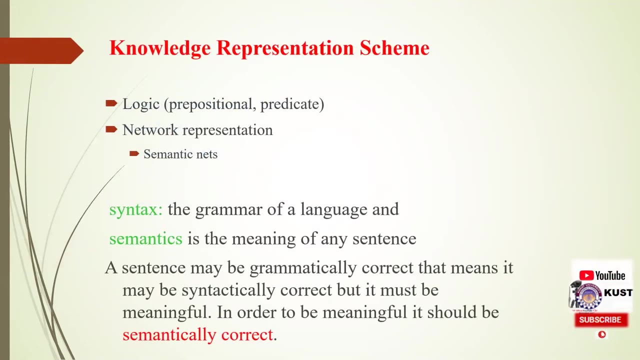 is the semantic network. We'll see what is the meaning of semantic network and we'll also talk about nodes and arcs in semantic network with examples. In the last lectures we have looked into different knowledge representation schemes, namely the propositional logic and first-order logic or predicate logic. Today we will start. 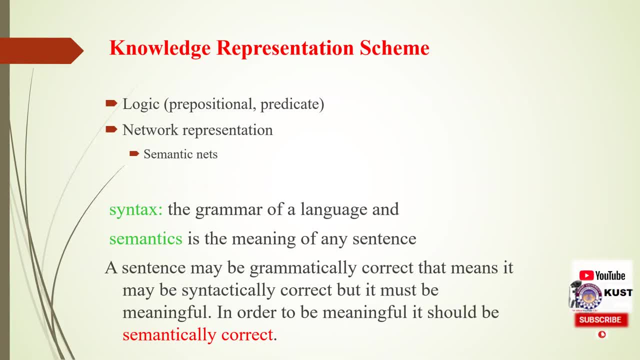 discussing on another mode of representation of knowledge, known as semantic nets. The word semantic means meaning. As a computer science student, you are already familiar with two words: the word semantics, which is essentially the grammar of a language, and semantics is the meaning of any sentence. So I may form the sentence correctly, which. 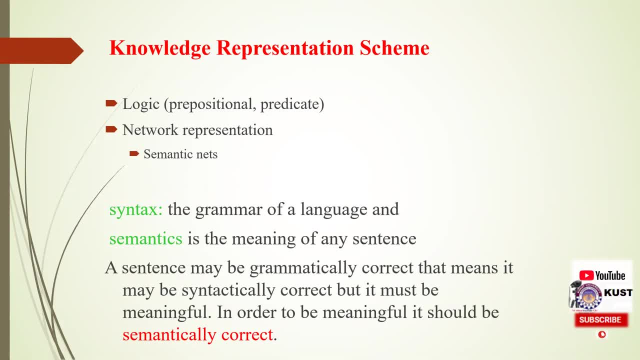 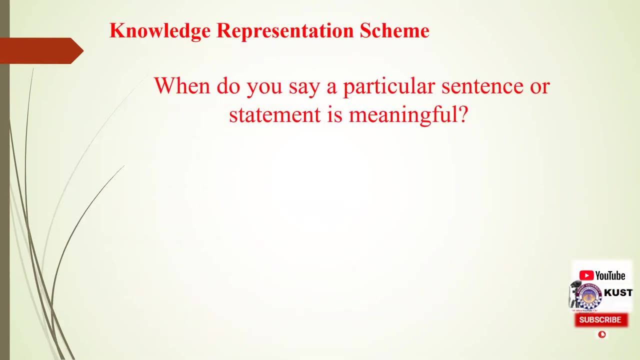 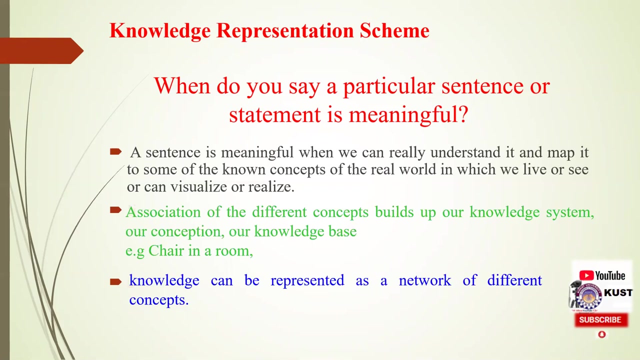 means. it may be syntactically correct, but it must be meaningful. In order to be meaningful, it should be semantically correct. When do you say a particular sentence or statement is meaningful? When there are no clearictions. it is important to have an effective meaning. Let's start with the sentence to the script. 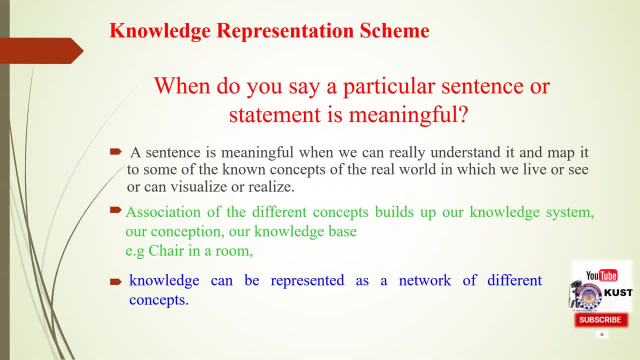 The sentence is meaningful when we can really understand it and map it to some of the known concepts of the real world in which we live or see or can visualize Whatever we look at. For example, If I look at this room, then I'll be looking at what is this room likely? to be like in reality. There are a lot of Picklebol to choose, such as. I just want to show you that somehow it makes sense to have a gender and have a gender identity. Now let's try to figure out which is the symmetry of this. 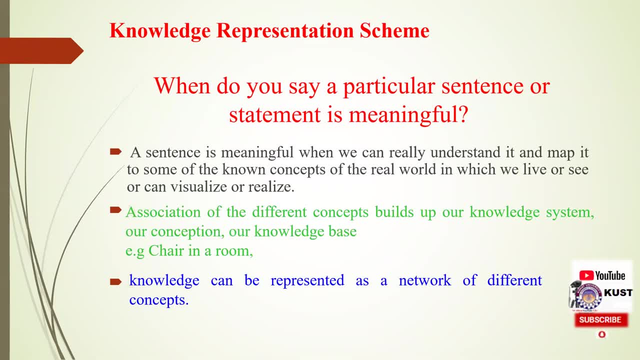 representation. So what happens if we pull this command line? We want the Wanhui character. there are a variety of keywords for it to be connected to the word semantics: different chairs, tables, etc. now, each of these are different concepts and the chair, for example, is made up of wood. there can be chairs which are not made. 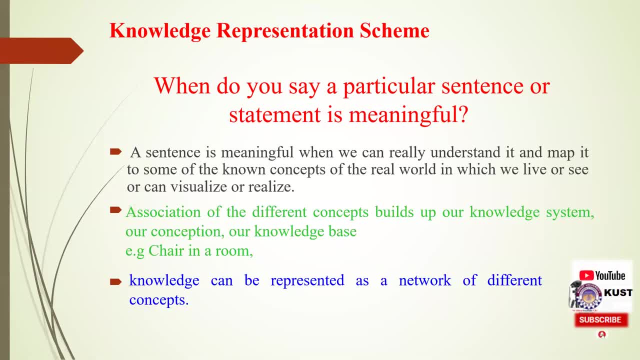 of wood that may be made of iron, steel or some other material. so whenever we talk of chair, we can think of some other associations related to the chair. similarly, whenever we use a word, say a boy, then it got so many other associations. a boy will be at most of, say, 18 years old. he will be having height. 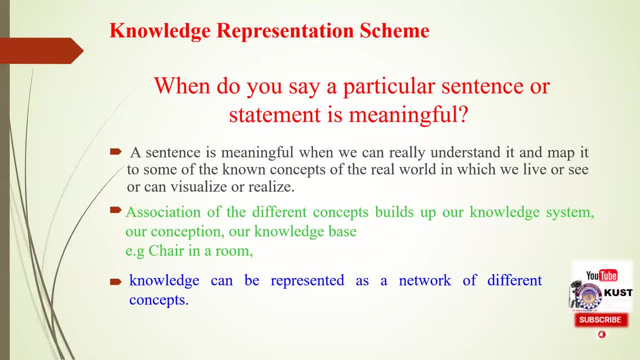 will be having weight and we may be going to school. so there are so many other associations that come up with a concept. so whenever we use any particular word, we are actually referring to some concept and along with that concept we immediately associate some other related concept. and this association of the different concepts. 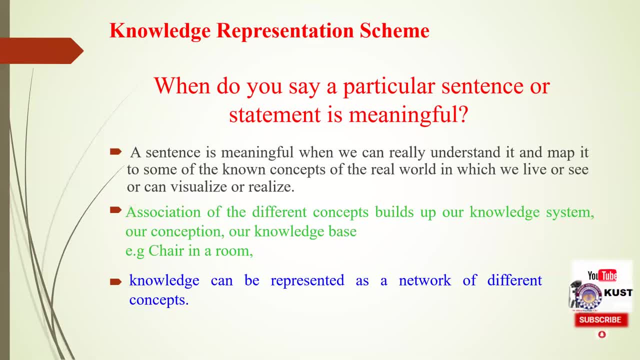 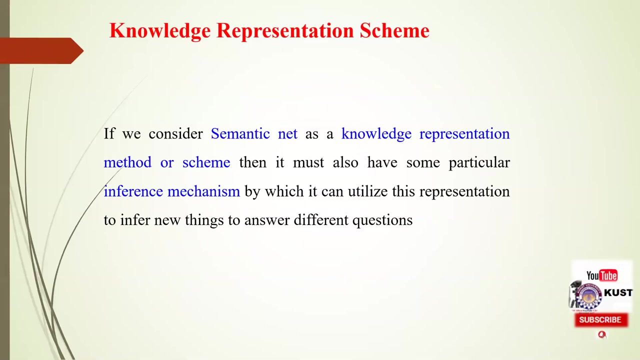 wills up a concept and this association of the different concepts wills up a knowledge system or our knowledge base. this is another view of looking at knowledge, that knowledge can be represented as a network of different concept. any collection of facts or information cannot be knowledge unless it is used. 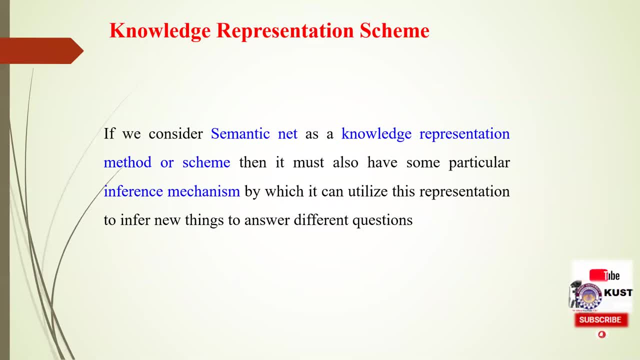 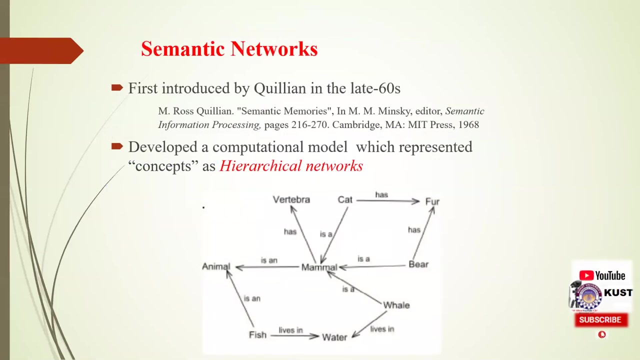 for inferring some new facts. if we consider semantic net as a knowledge representation scheme, then it must also have some particular inference mechanism by which it can utilize this representation to infer new things to answer different questions. the idea of semantic nets dates back to 1966 in two very important papers that 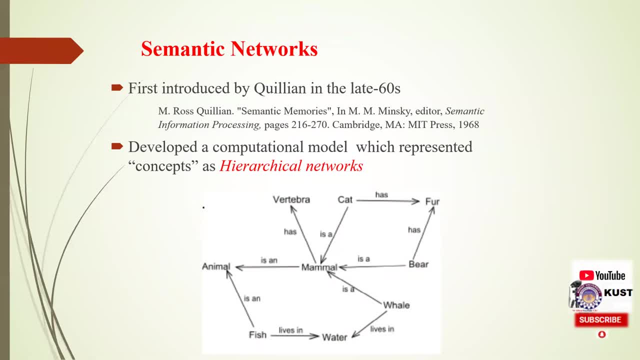 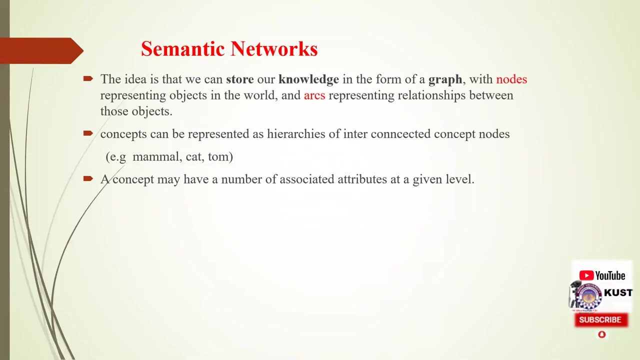 were written by Rose Quillen, who was one of the early working developers of artificial intelligence. he tried to represent the organization of human semantic memory, or knowledge, as a hierarchical network. it is used for analyzing meanings of words within sentences. semantic network is simple representation scheme which uses a 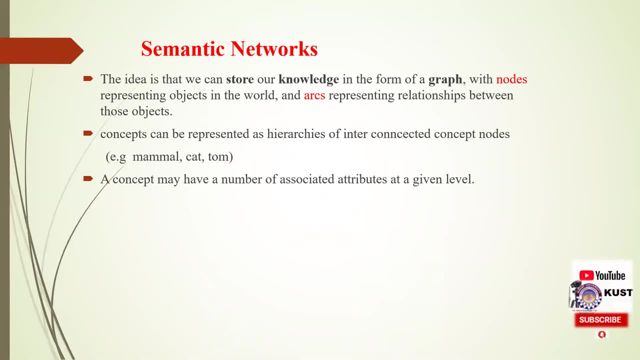 directed graph consisting of nodes which represent concepts and directed arcs to which represents semantic relation between the concepts. in this, concepts can be represented as hierarchies of interconnected concept nodes. for example, it is very natural to draw the link between cats and animals, to say that cats are animals. 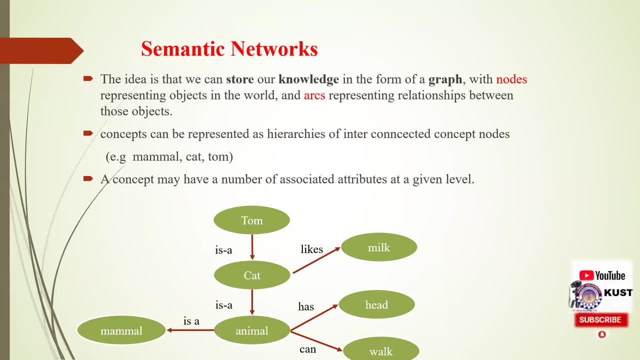 a concept may for a number of associated nodes, their links with a public, and I attributes at a given level animal has had. an animal can walk. this is one level. cat is on another level where there is another association attached to it: cat likes milk. this association is not related with all the with all animals. 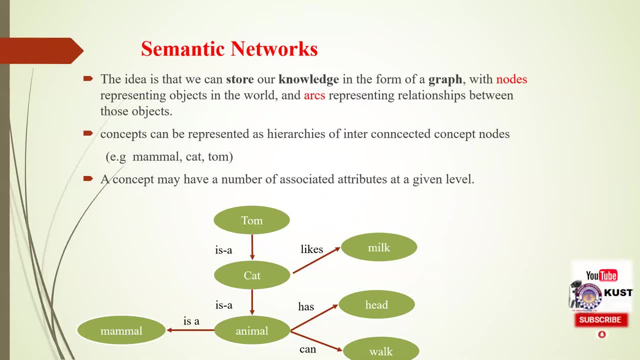 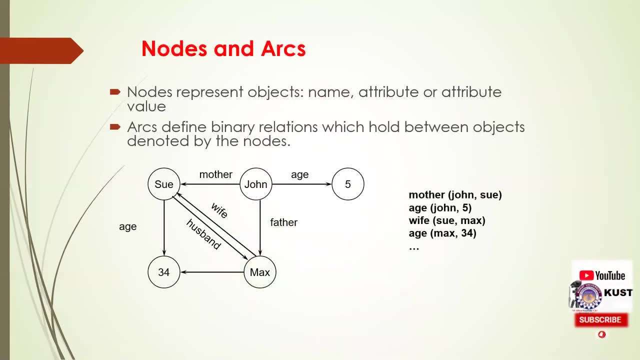 this is in this graph. it is only associated with the cat. nodes in the semantic network represent objects that may object may be named attribute or any attribute value, and the arcs are links, define binary relations which hold between objects denoted by the node on the right side. on the right, there is a propositional logic in front of which 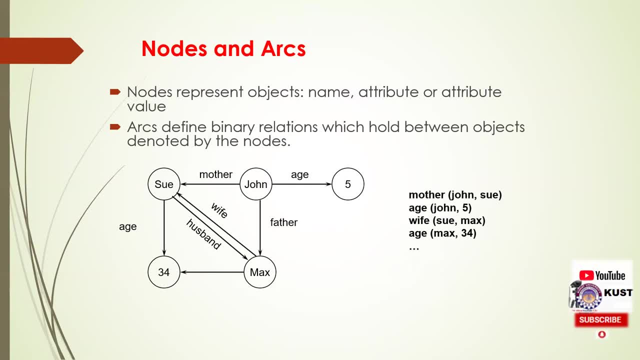 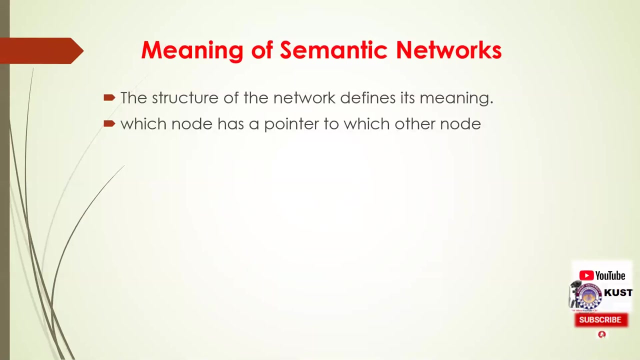 is the equivalent semantic nets, where the nodes represents the objects and their links are the predicates that are in the propositional logic. the structure of the network defines its meaning. the meanings are merely which house which node has appointed to which other node. the network defines a set of 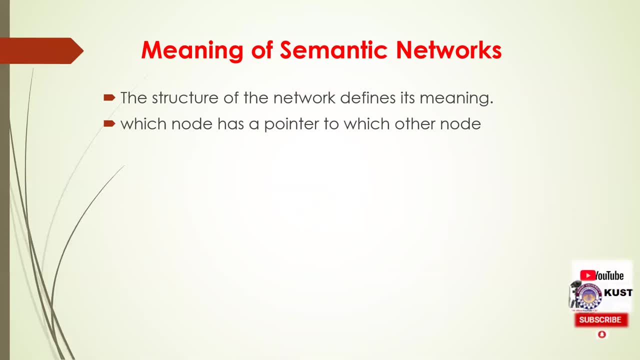 binary relations on a set of nodes. to begin, simply, let us introduce two nodes and a link. a particularтерA is a string line, a particulartaterA is a link with no other идеas as linked in the Godsars Bill market. The node on the right, labeled can't, is linked to the node on the left. 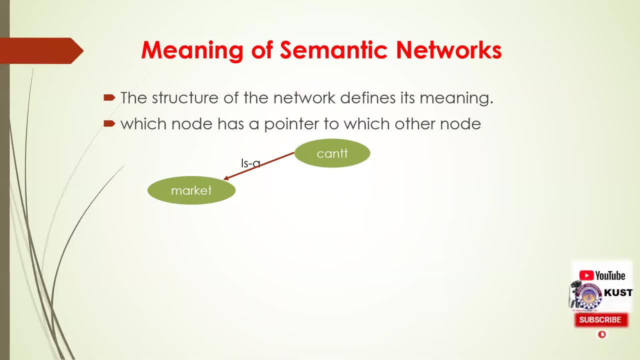 labeled market and the arrow is labeled is a Can't is an example of a market. The diagram, in other words, represents the fact that there is a wider relation between a market can't and the concept of a market. Another node with the label Rajabazaar and is a link from this node to the market node could be added again. 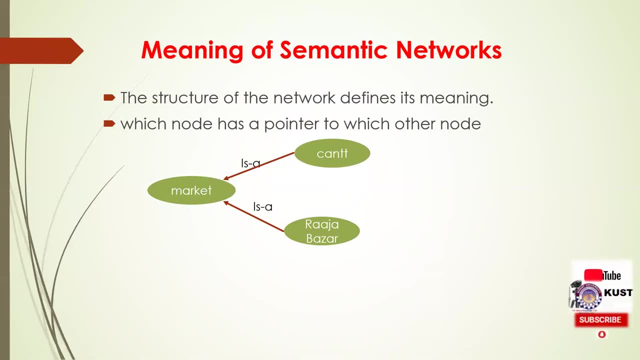 representing that Rajabazaar is a type of market. If a retailer node is added to this figure, the structure of the network becomes as Markets generally contain retailing entities. To add an example of a retailer, we add a node labeled Ahmedabad, Ahmedabad garments and two links, one from the retailer Ahmedabad garments to Rajabazaar. 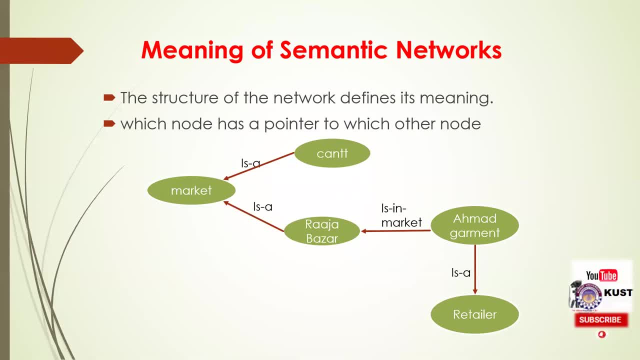 labeled is a and one from the node Ahmedabad garments to the node retailer. This illustrates that Ahmedabad garment is a retailer in the Rajabazaar. Now it is important to note that the retailer is a retailer in Rajabazaar. Let us emphasize that the node labeled market represents the generic or meta concept of a. 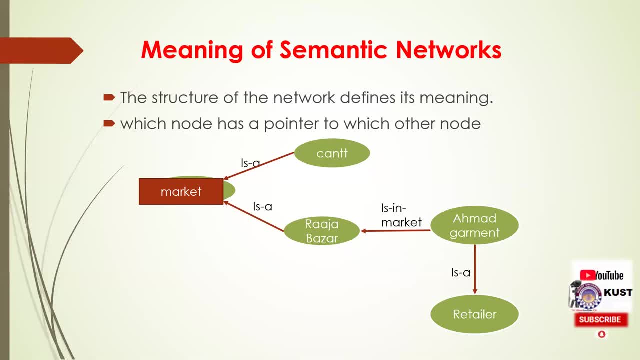 market. It came in thought of as possessing photographers common to all markets. Theð Nó Ariana was a represents a particular market. The note retailer again represents the same concept Of a retailer that is common in a particular market, more probing than a main market. 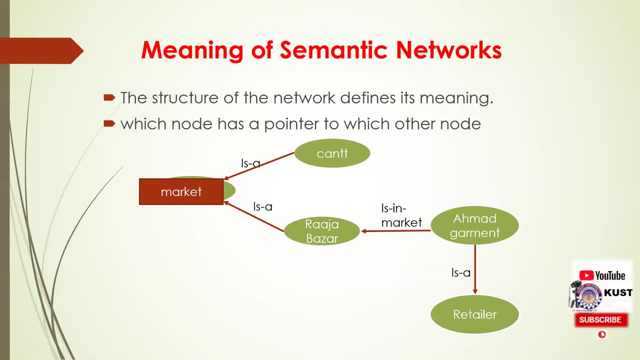 to sell products in the market. that is generalizing or unnecessary. Now we are going to study a topic called 했a Ukraine: avilion of some details. A market is a marketä, the concept that is. there come so many treatment. many states and economic practice must notice their customer of those traits. 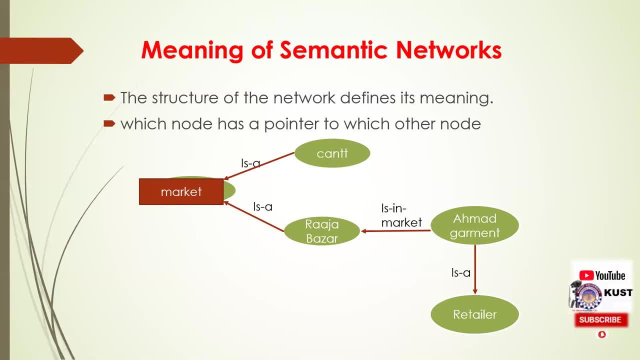 all the enrollment of the business. let'siza thebe seems Sáhe be nine. once morePHD your desires. it is Raja Bazaar that is common to a seller across all particular retailers, and Ahmed garment is one instance of such a retailer. 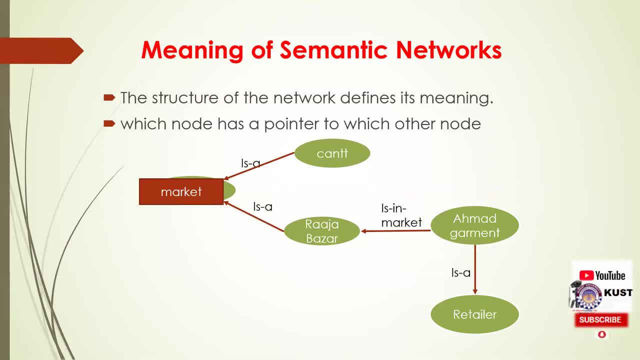 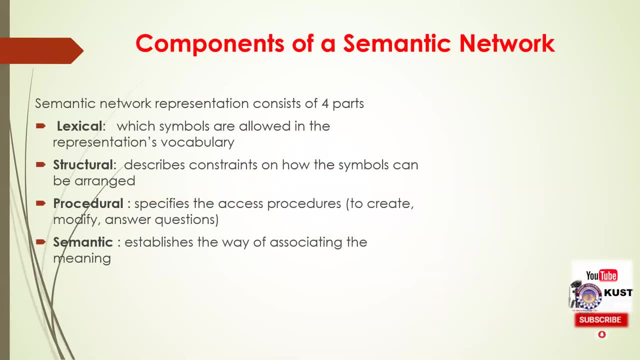 We can distinguish the two types of nodes using boxes and circles. Link network representation consists of four parts. The lexical part includes nodes, arcs or links and their labels. The structural part shows that how the links and nodes form a directed graph. The procedural part specifies the access, the SS procedures, that is to create a network. 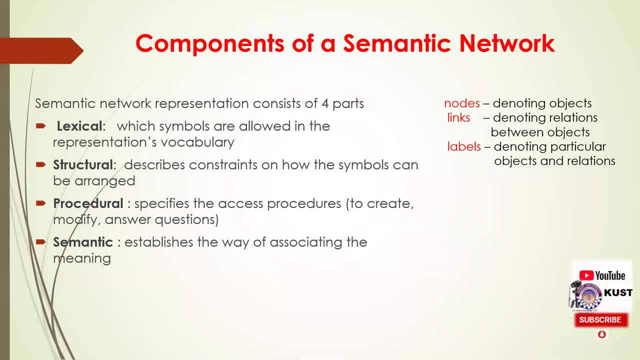 to create, modify the nodes and to generate answer questions. If constructor is a procedure, then it will allow creation of new links and nodes. Similarly, if destructor or modify is a procedure, then it will do their work. Modifier will modify the nodes and the destructor will allow to delete the links and nodes. 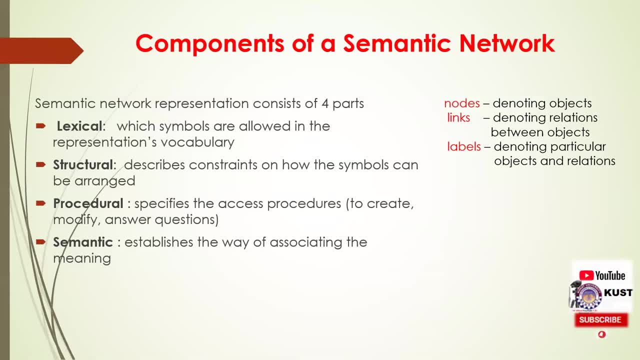 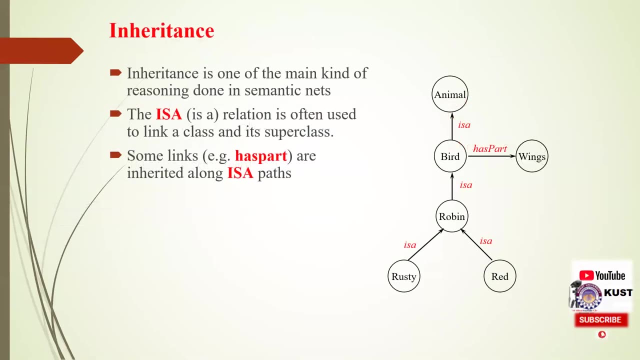 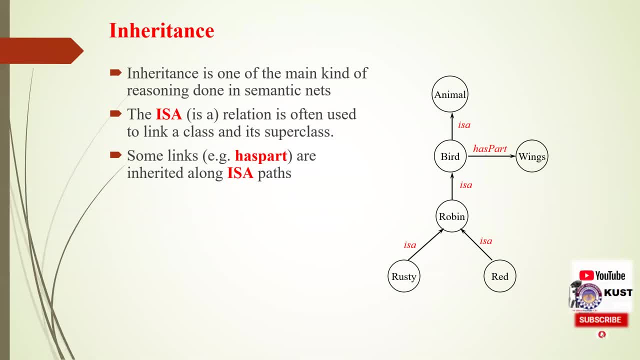 The idea of this is that if an object belongs to a class, it inherits all the properties of that class and can be represented by is a link In general. if concept X has property P, then all concepts that are a subset of X should. 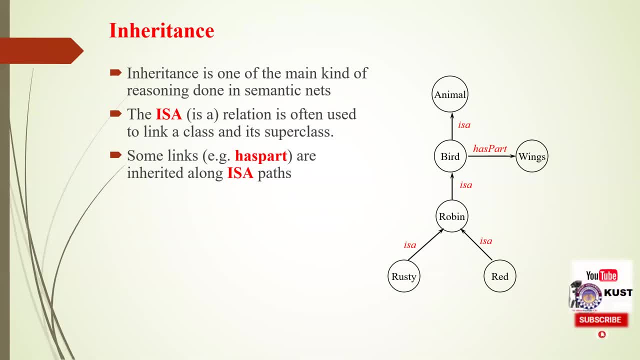 also have property P. In this example we can see that a subset of Y equals P. In general, if concept Z represents E, then every element in the And then in this example, the property as a subset equals P, then all concepts are unable to be represented by an un disposeds project at any moment. on the layout. Therefor, for the sake of simplicity, we need to remember first that even in practice lettering that we have, there are different types of verb owners. In our case there are two types of verb owners that, in nervously repeat after eachim, not HAVE the twenty components. 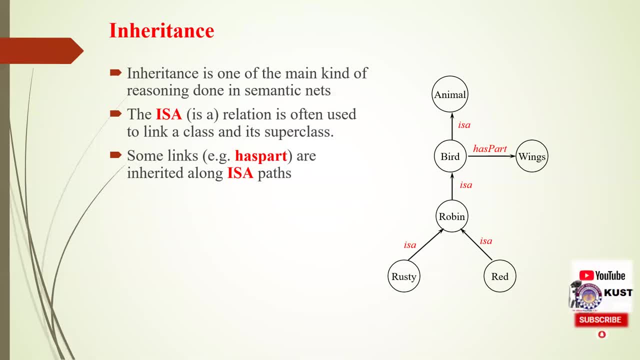 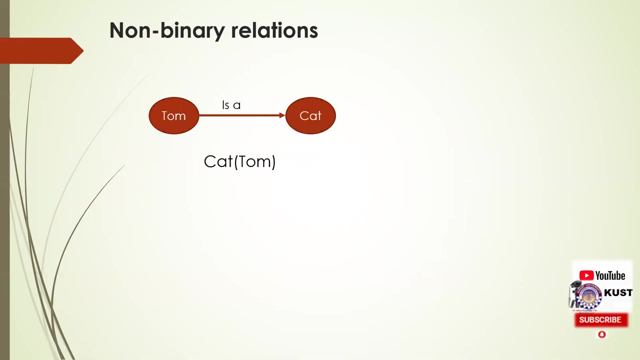 There's thathave both nationales firmatistic characters, which is W Environment, And also Hassrodic we'll talk about. mutatern and red must have wings because they inherited this property from their superclass. Non-binded relations. We have seen how binded relationships may be represented by arcs and 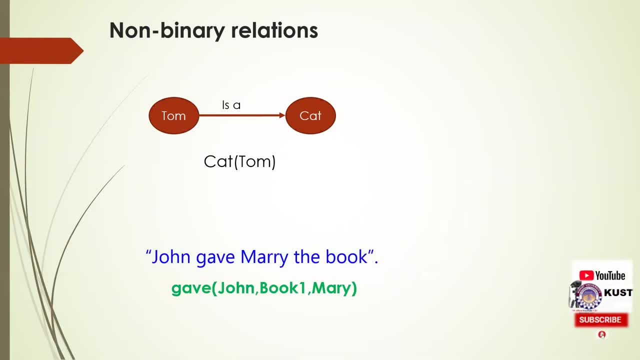 by arcs in the semantic nets. But what about relationships with more than two arguments? For example, how we can represent the sentence John gave Mary the book in the semantic networks? In predicate logic we could have a three-day predicate give whose first argument is the 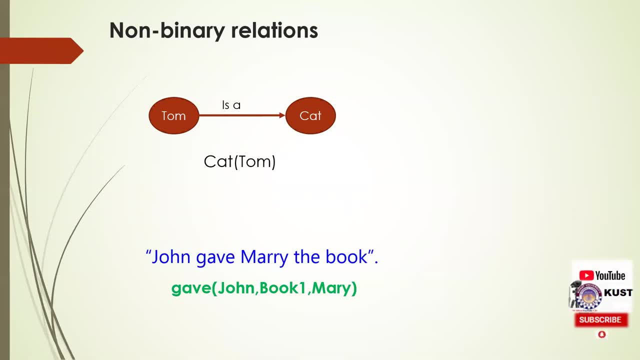 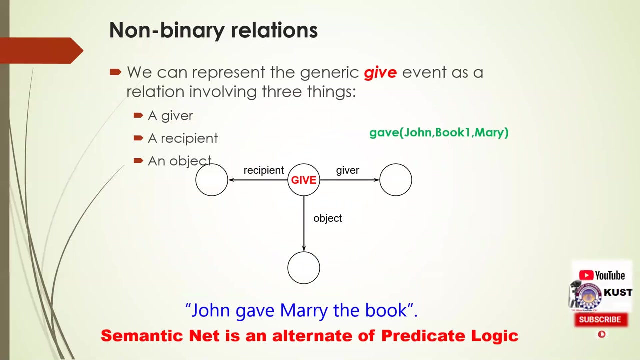 giver. Second argument, the object that is given. and third argument is the person to whom it was given. This way this can be resolved is to consider the act of giving a separate object. We can represent the generic give event as a relation involving three things in the semantic network: A giver, a recipient. 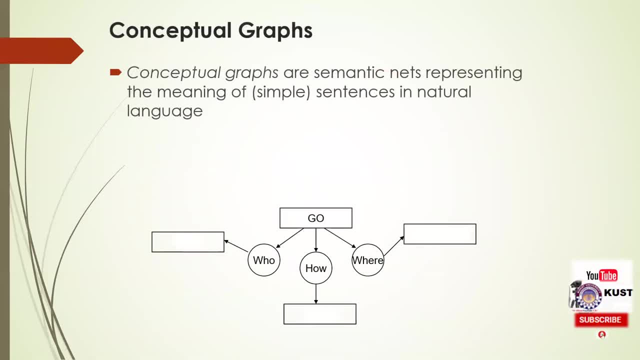 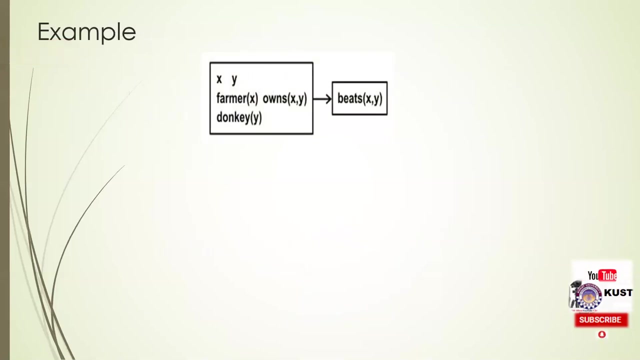 and a recipient. This is also known as conceptual graph. Conceptual graphs are semantic nets representing the meaning of sentences in natural language. Another example of conceptual graph is can be seen in this graph: John goes to New York by bus. This is an example of propositional logic. If a farmer owns a donkey, then he beats. 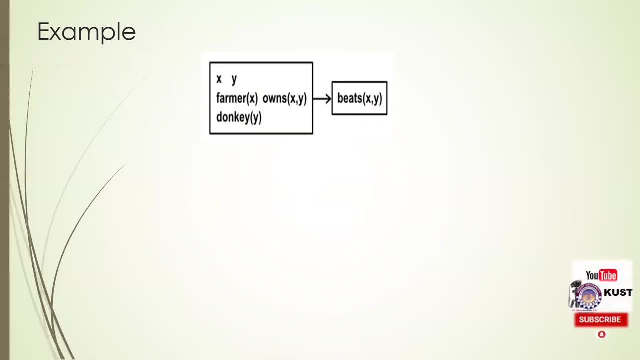 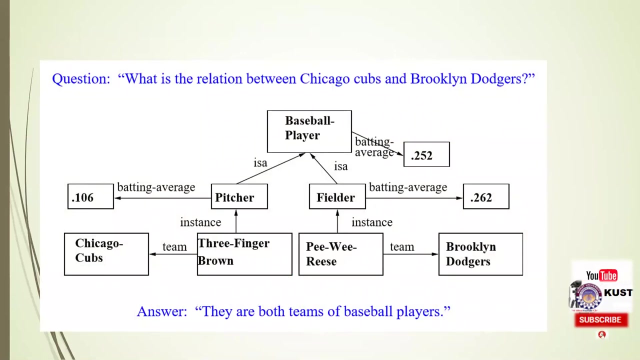 it. This can be converted into a semantic net as: And this graph can again be translated to the following predicate: logic Reasoning: investigationält 사랑. into graph matching, a question network is generated for each question. we get an answer when the question network match to a sub graph of the semantic network. 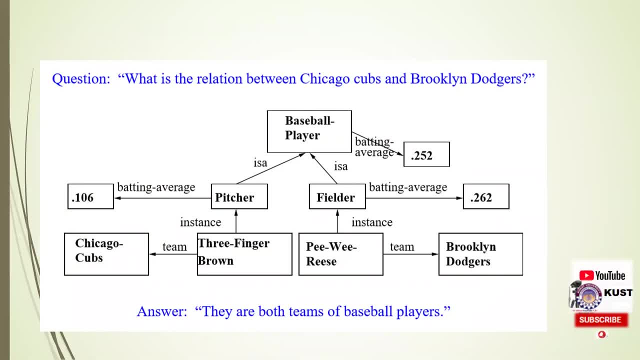 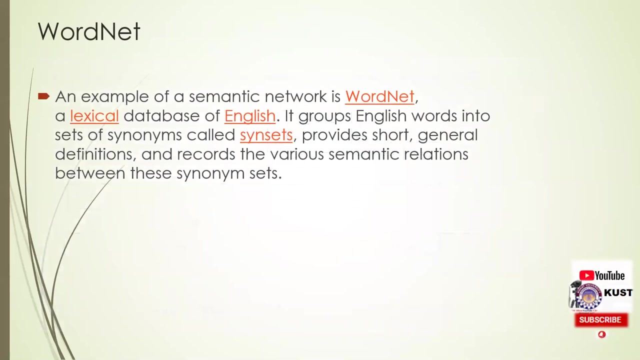 if the graph is given and a question is asked, then following the links between the nodes one can deduce the answer. so this is an example of how answer can be generated using semantic networks. just follow the links and nodes and conclude the answer. WordNet is an example of a semantic network which is a lexical. 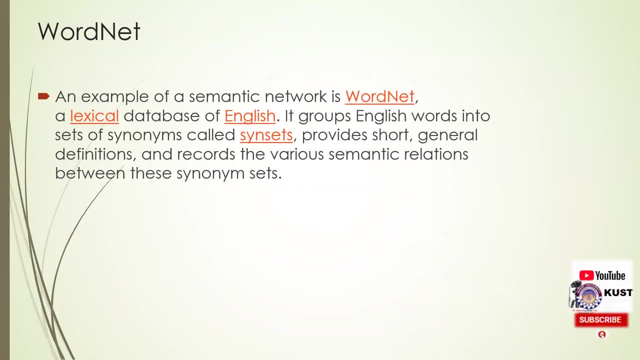 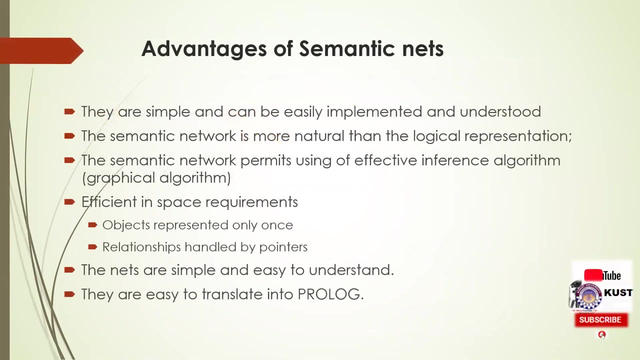 database of English. it groups English words into a semantic network and then sets of synonyms called since sets, provides short general definition and records the various semantic relations between these synonyms sets. these are some of the advantages of semantic networks. they are simple and can be easily implemented and understood. the semantic network is more natural. 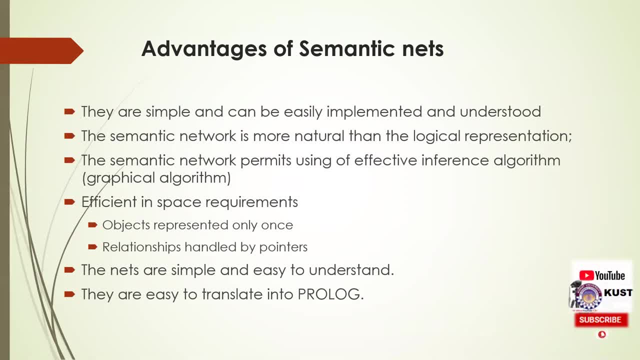 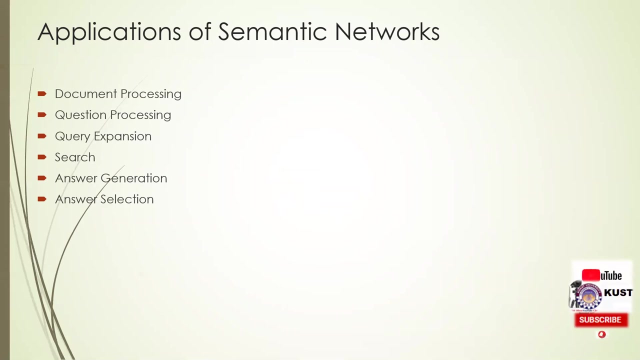 than the logical representation of a semantic network. it permits using of effective graphical algorithms. they are efficient in space requirements as objects are represented once and the relationships are handled by pointers. they are easy to translate into prologue and nowadays, in python. some of the applications of semantic networks include document processing, question processing and 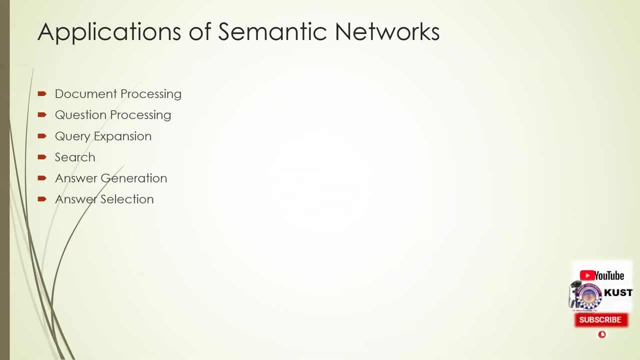 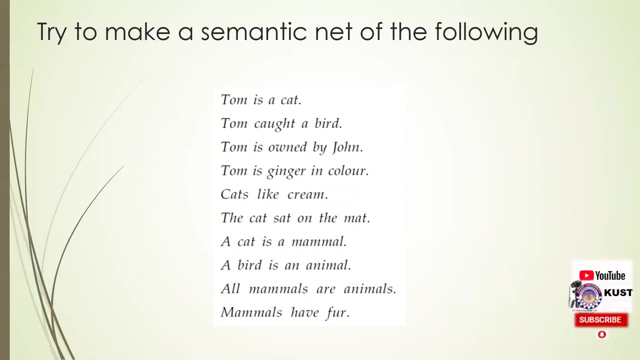 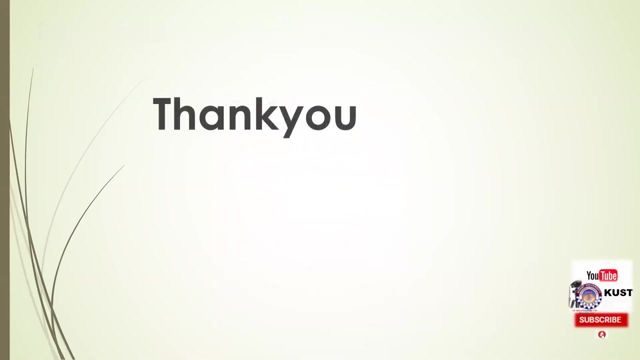 processing query expansion. We can use semantic networks in searching. It can be used in answer generation and answer selection. Students are encouraged to make a semantic net of the following: Thank you,